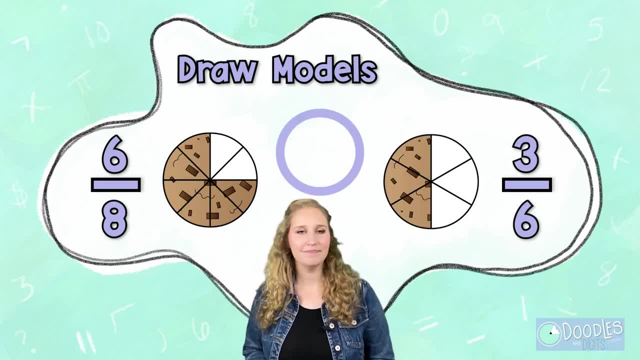 us compare fractions. Let's look at these two fractions here. What do you notice? Which one is greater? That's right. We can actually look at visuals or models to help us compare fractions. Let's try a few more. Let's try these two. 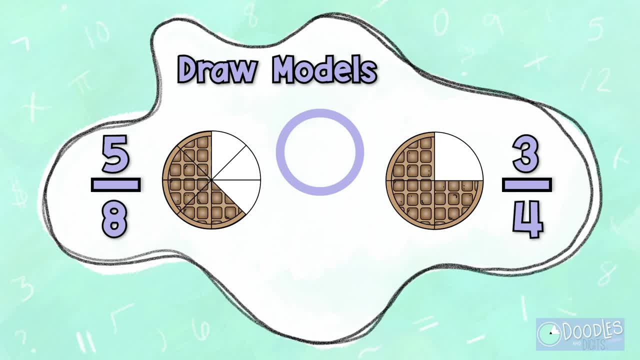 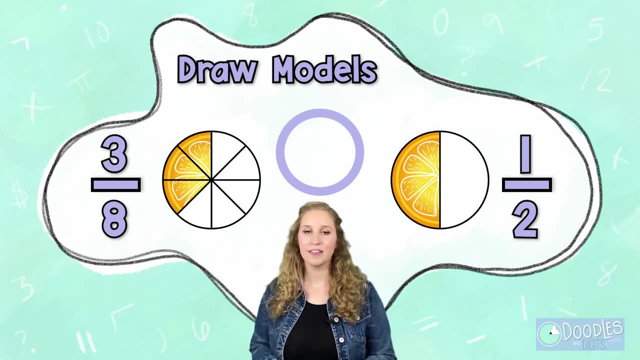 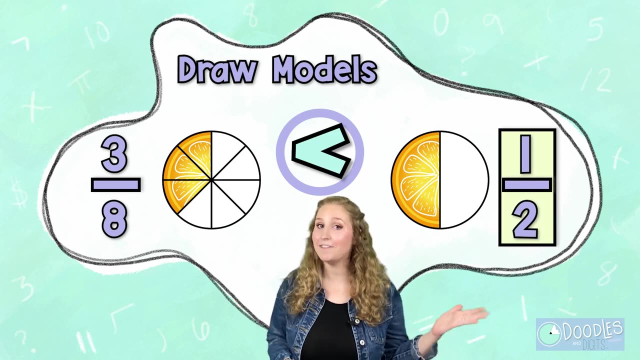 Five-eighths or three-fourths, That's right. All right, let's look at one more. Three-eighths or one-half. Yeah, these actually have different denominations. They have different denominators, but you can easily see with the visual which one is greater. 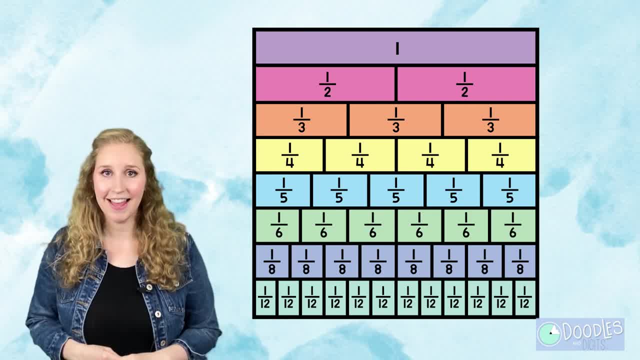 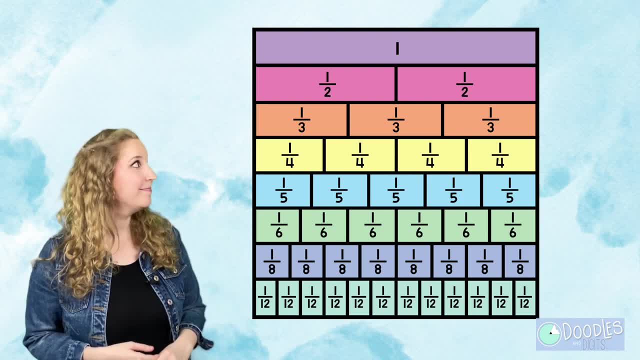 You can also use a fraction chart to help you compare fractions. Let's look at this fraction chart here. All right, what do you notice about the fraction chart? Let's try comparing two numbers. Which one's larger, One-half or two-fifths? 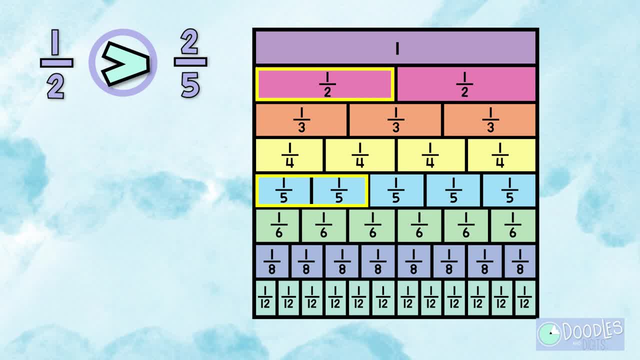 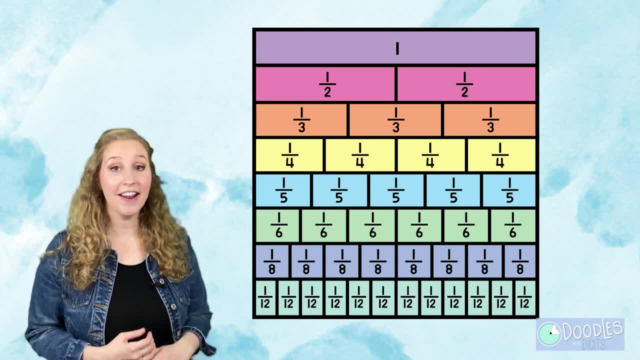 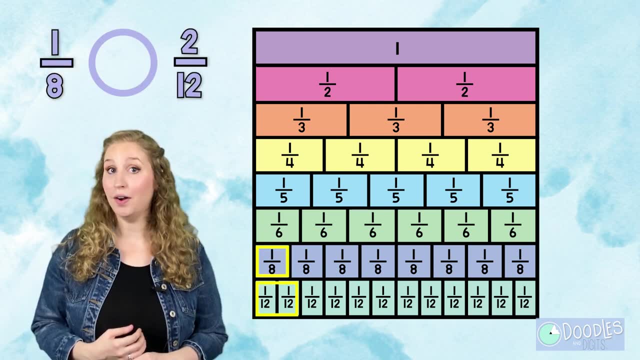 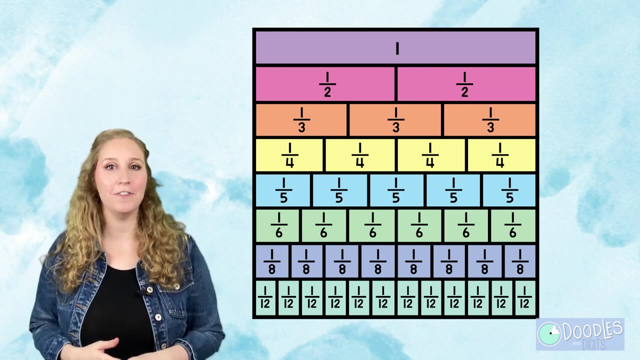 By looking at the chart you can see that one-half is greater than two-fifths. All right, let's try another one. Which one's larger, One-eighth or two-twelfths? Now that we've tried a few together, let's see if you can compare a few on the number chart right now. 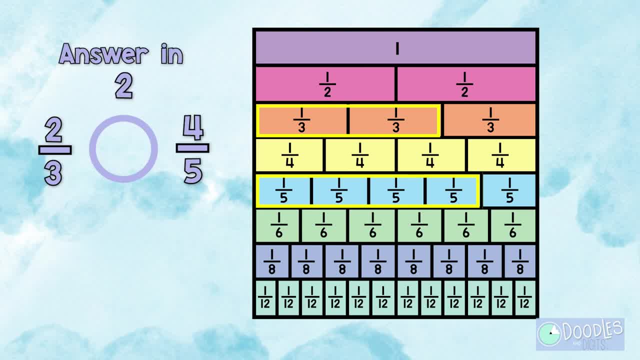 Two-thirds or four-fifths. Two-thirds is less than four-fifths, Four-sixths or ten-twelfths. Four-sixths is less than ten-twelfths, Five-eighths or three-fifths, Five-eighths is greater than three-fifths. 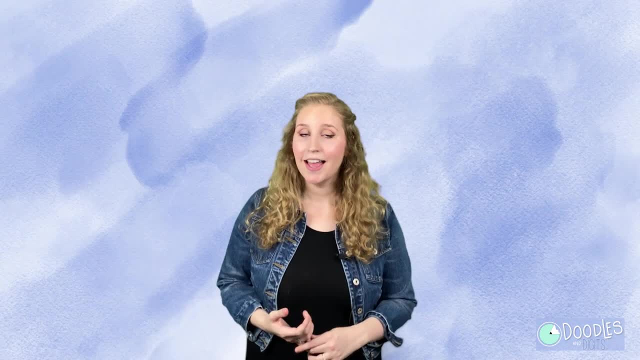 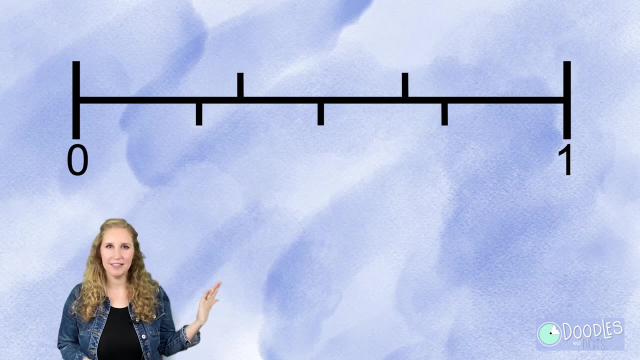 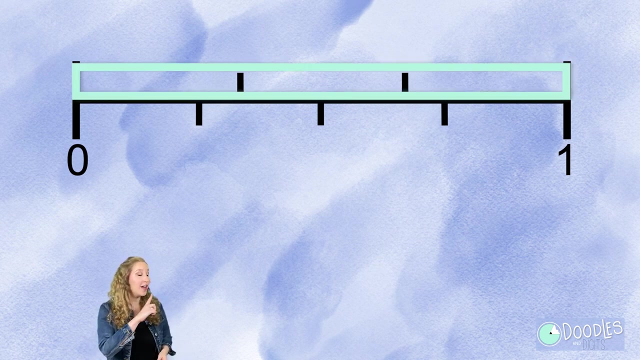 A number line is another great tool to compare fractions. Let's look at a number line. A number line, Alright, what do you notice? What's going on with this number line? Yeah, you might notice that there's actually a different fraction being shown on the top of the number line. 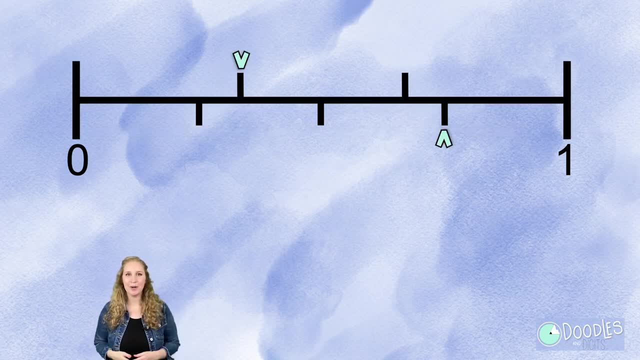 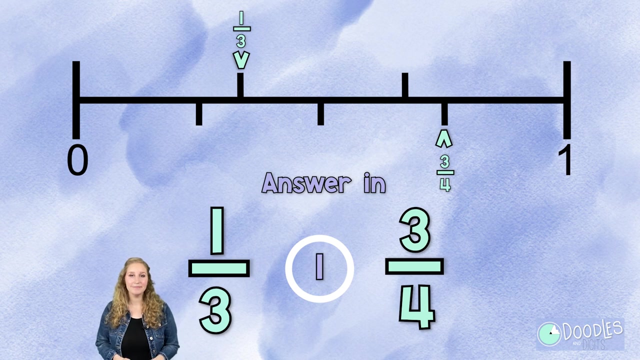 than the bottom of the number line, What two fractions are being shown. So when we compare fractions, we can actually place both fractions on this same number line to compare them. Let's try these two fractions. Which one's greater? all right, let's try another one. let's compare these two fractions with the number line two. 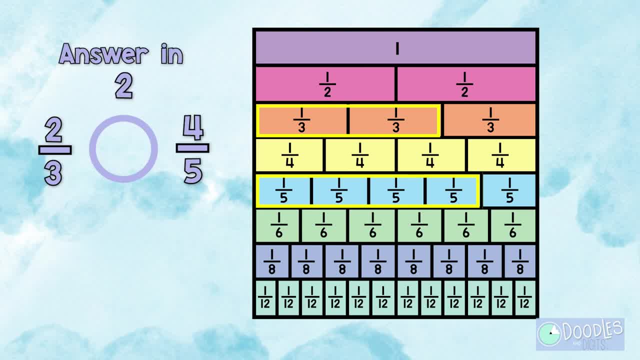 Two-thirds or four-fifths. Two-thirds is less than four-fifths, Four-sixths or ten-twelfths. Four-sixths is less than ten-twelfths, Five-eighths or three-fifths, Five-eighths is greater than three-fifths. 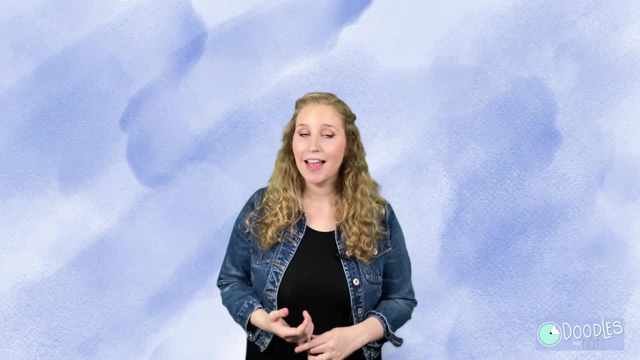 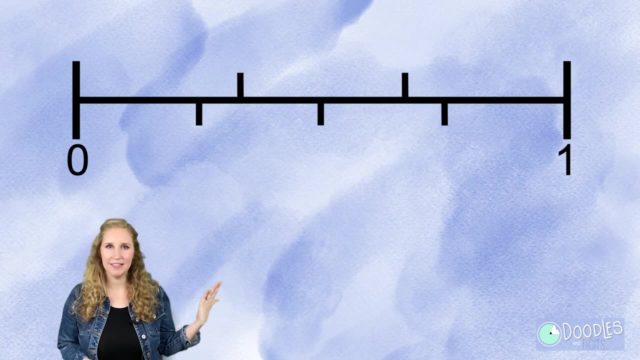 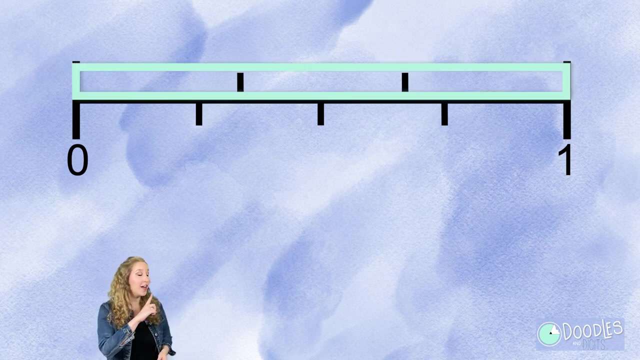 A number line is another great tool to compare fractions. Let's look at a number line. A number line. All right, what do you notice? What's going on with this number line? Yeah, you might notice that there's actually a different fraction being shown on the top of the number line. 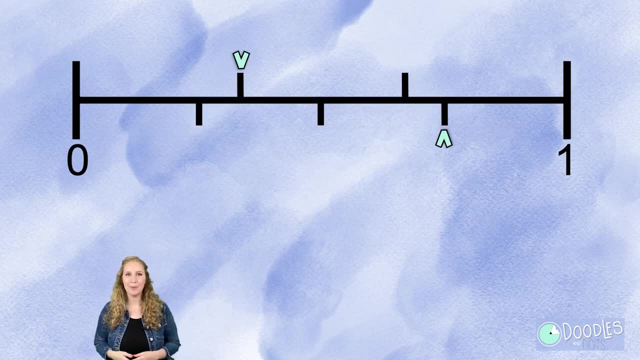 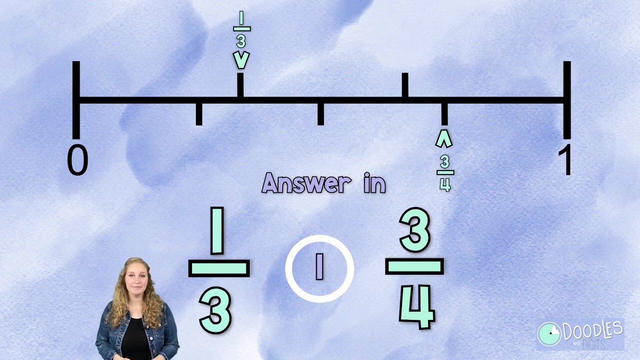 than the bottom of the number line What two fractions are being shown. So when we compare fractions, we can actually place both fractions on this same number line to compare them. Let's try these two fractions: Which one is greater? All right, let's go. 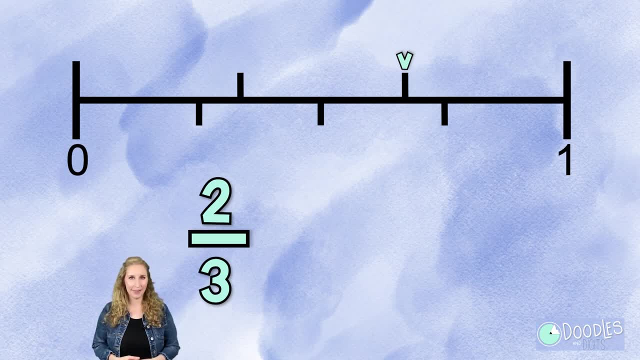 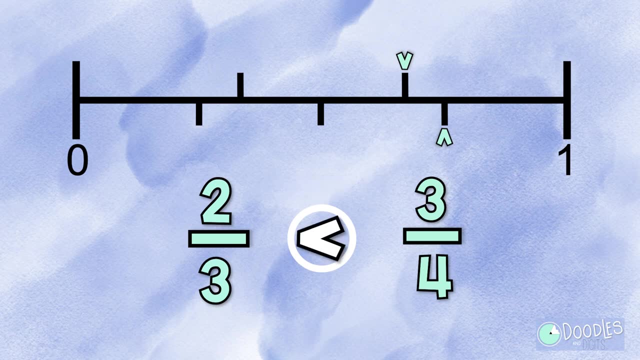 Let's try another one. Let's compare these two fractions with the number line: Two thirds and three fourths. Two thirds is less than three fourths. All right, now that we've tried a few together, let's see if you can compare a few fractions. 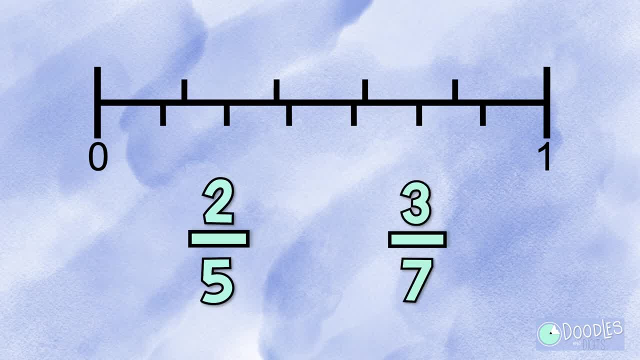 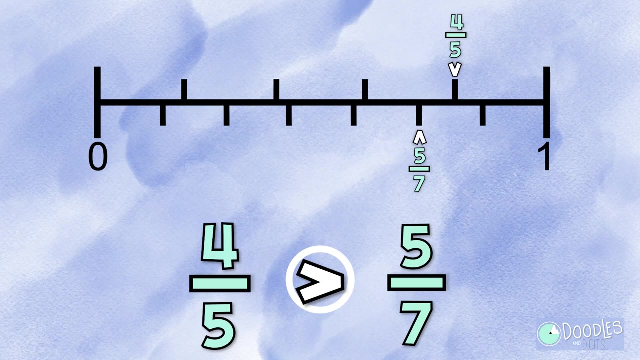 using a number line on your own: Two fifths and three sevenths. Two fifths is less than three sevenths. Four fifths and five sevenths. Four fifths is greater than five sevenths. The last strategy is: you can also use reasoning. 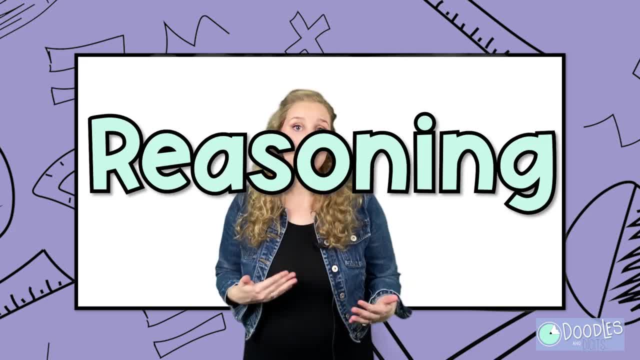 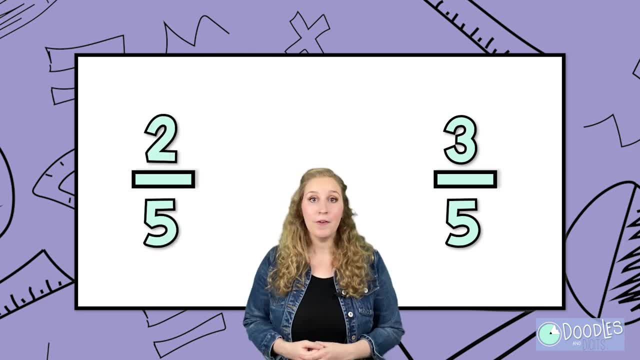 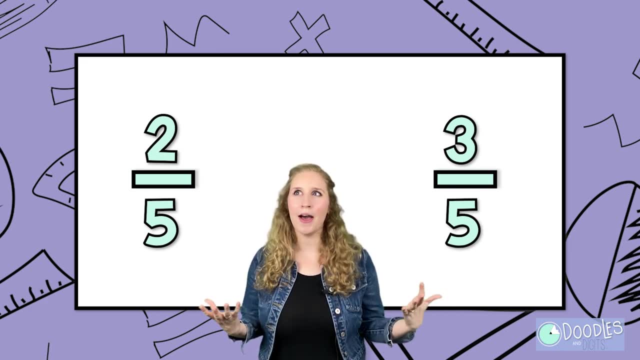 to compare fractions. So, for example, you can actually use benchmark fractions and then just looking and thinking through it to know which one's greater. So, for example, if we're looking at these two fractions here, they both have the same denominator. So we can think: what do I know about this? 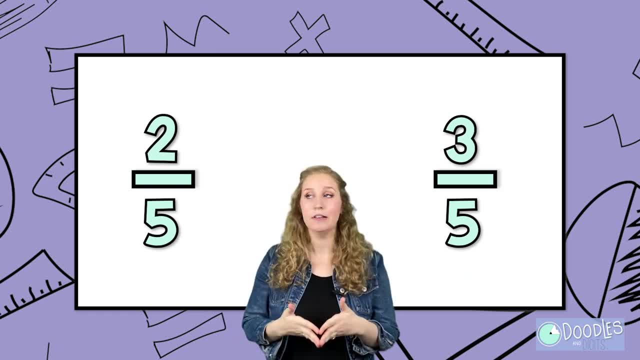 Well, we know, if you have the same denominator it's the same size piece. So whichever one has more pieces is going to be greater. Let's look at this here. You've got two fifths and three fifths. They both have fifths in the denominator. 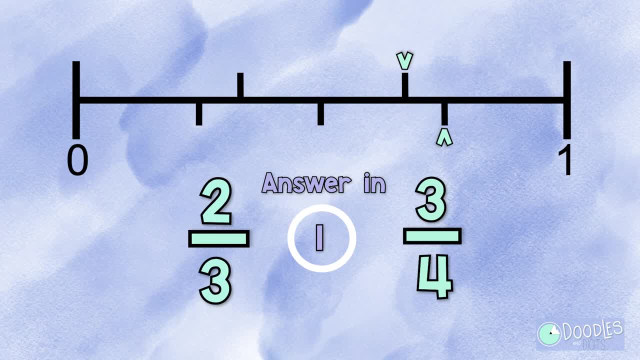 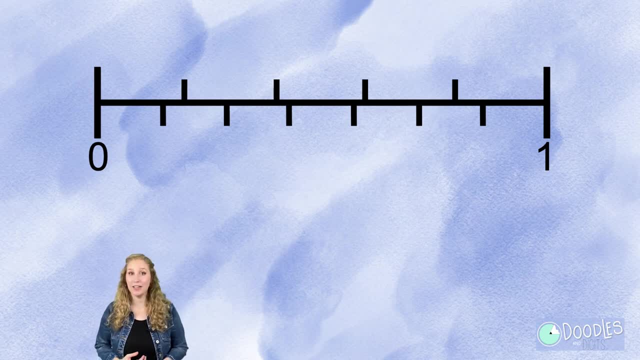 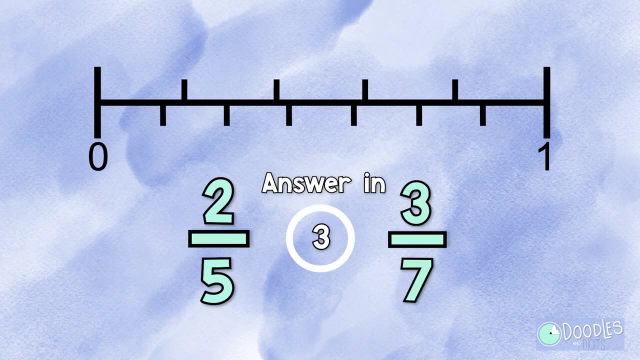 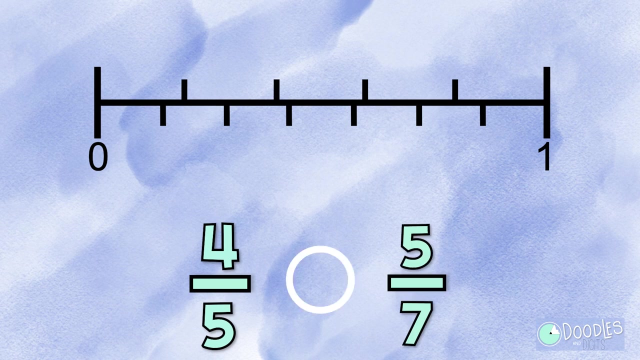 thirds and three-fourths. two-thirds is less than three-fourths. all right, now that we've tried a few together, let's see if you can compare a few fractions using a number line on your own. two-fifths and three-sevenths. two-fifths is less than three-sevenths. four-fifths and five-sevenths. 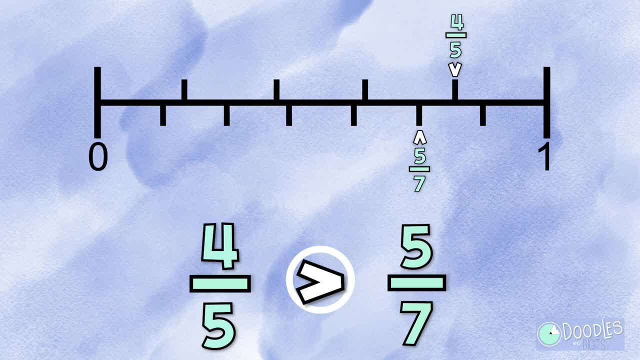 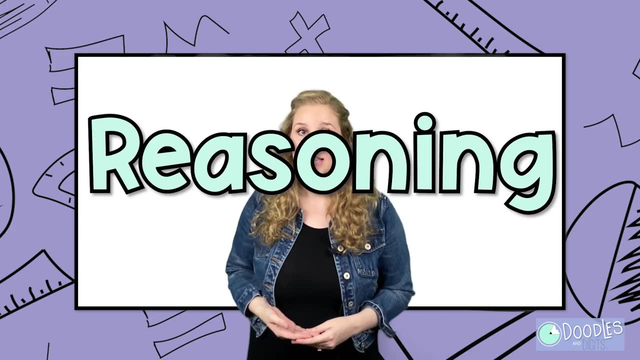 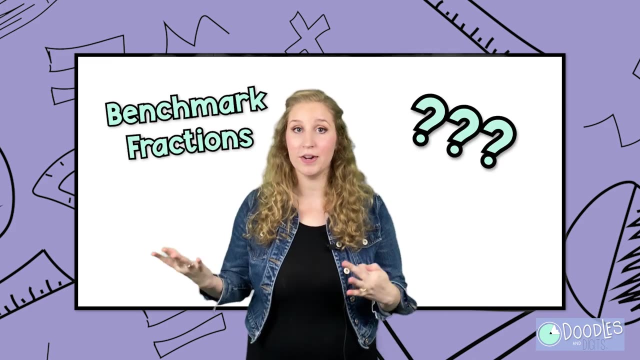 four-fifths is greater than five-sevenths. the last strategy is: you can also use a reasoning to compare fractions. so, for example, you can actually use benchmark fractions and then just looking and thinking through it to know which one's greater. so, for example, if we're looking at these two fractions here, they both have the same denominator. 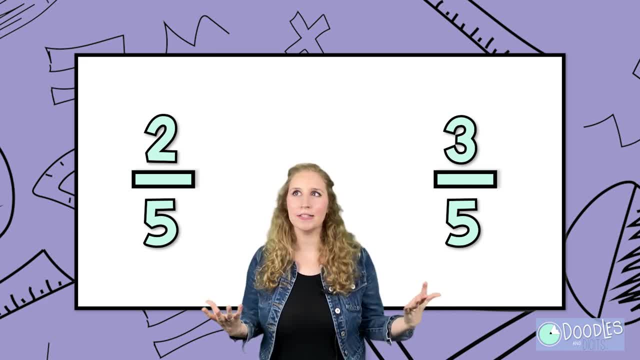 so we can think: what do I know about this? well, we know, if you have the same denominator, it's the same size piece, so whichever one has more pieces is going to be greater. let's look at this here. you've got two-fifths and three-fifths. they both have fifths and the denominator, so we can. 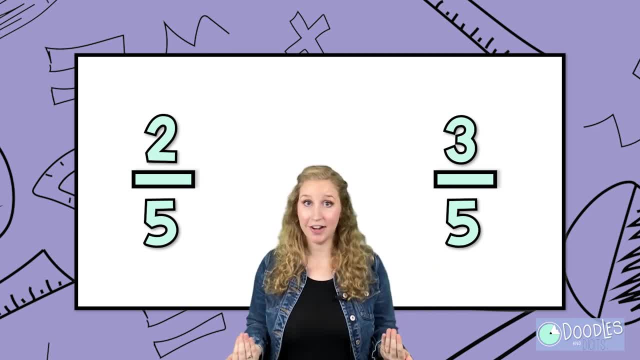 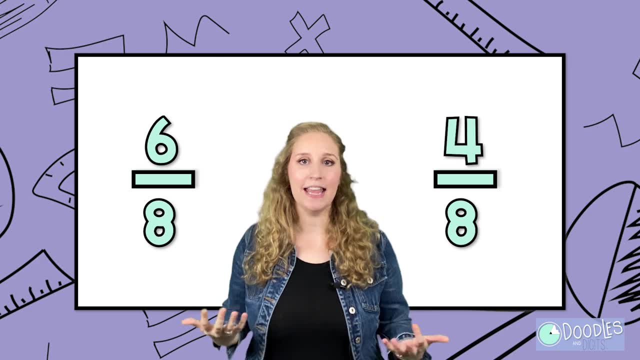 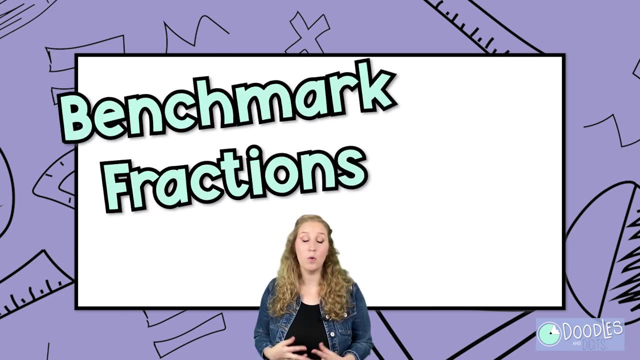 look at the numerator and know that the three-fifths is greater. let's try another one. what about four-eighths and six-eighths? since they have the same denominator, we know that the larger numerator is going to be greater. you can also use benchmark fractions like: 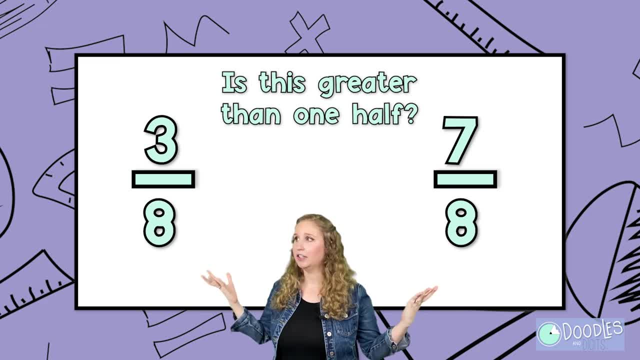 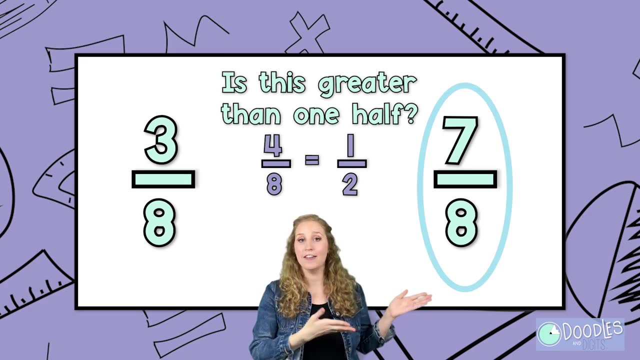 one half. so let's say we have these two fractions here. you can think, okay, is this greater than one half or less than one half? this one here is greater than one half, this one over here is less than one half. so we know, the one that will be greater than one half is going to be greater review. 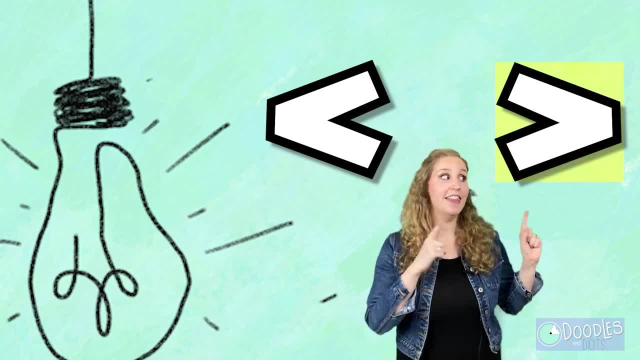 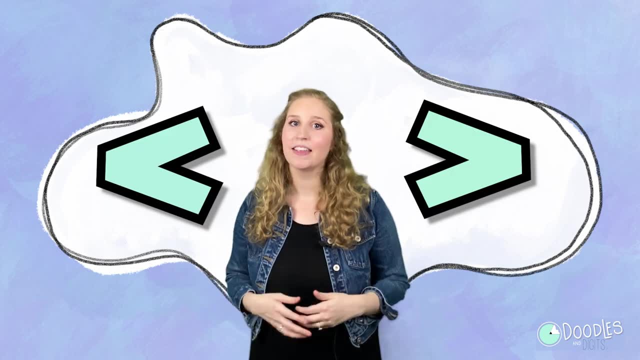 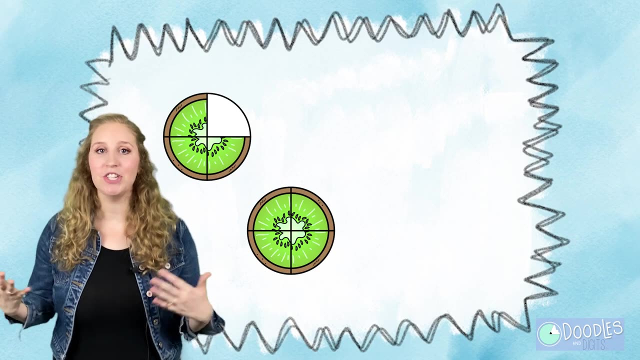 time. what is the greater or less than symbol? this is the greater than symbol and this is the less than symbol. how can you remember which one's greater than or less than? some people like to think of the opening as a mouth and eat the bigger number. now that we've learned a bunch of different. 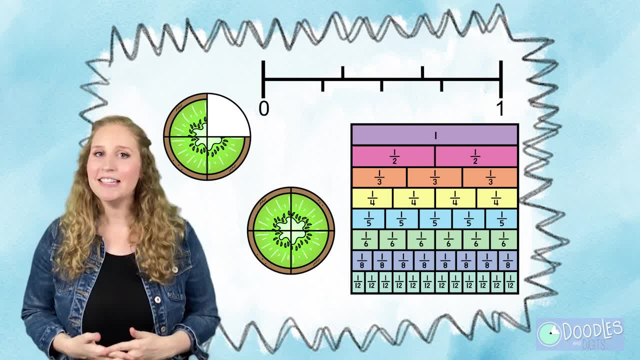 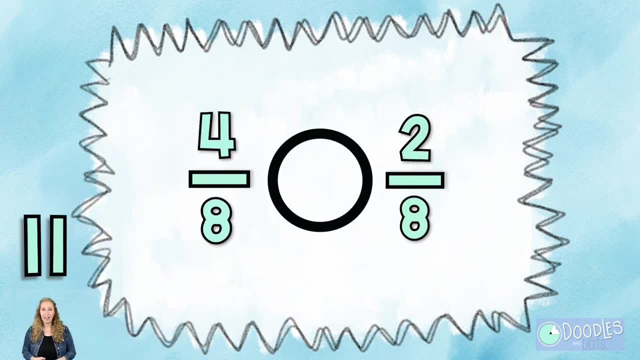 strategies and also we've done a few together. let's see if you can solve these on your own. you can use whatever strategy works best for you. remember you can pause this video in case you need more time. four-eighths or two-eighths. four-eighths is greater than two-eighths.